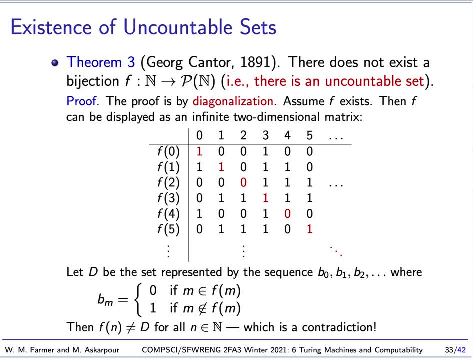 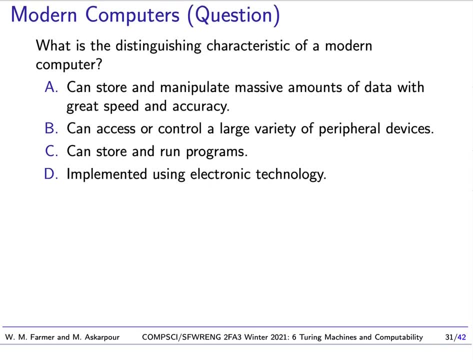 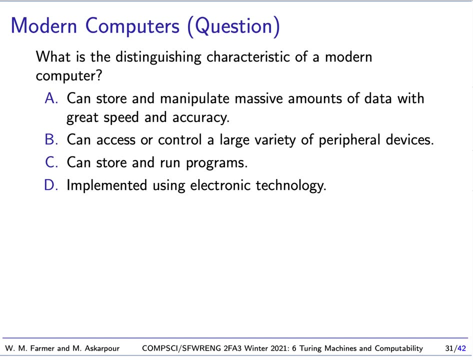 there is a particular problem, a particular decision problem that is undecidable. Now, a bit back, we had this question about modern computers: What is the distinguishing characteristic of a modern computer? And our answer is that modern computers can store and run programs. And if you think of a Turing machine as being as 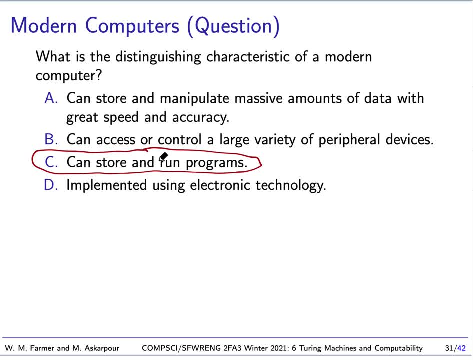 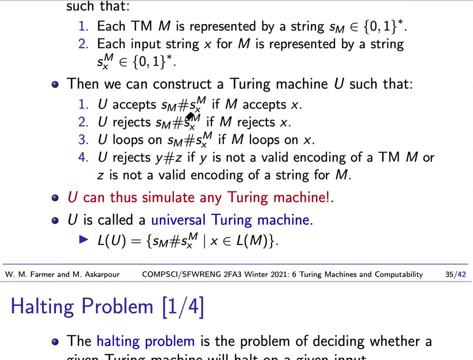 powerful as a computer and in some ways more powerful because it has infinite amount of memory. we should be able to store and run programs. So this brings us to the notion of a universal Turing machine. So what is a universal Turing machine? Well, we have to start off with. we need we're. 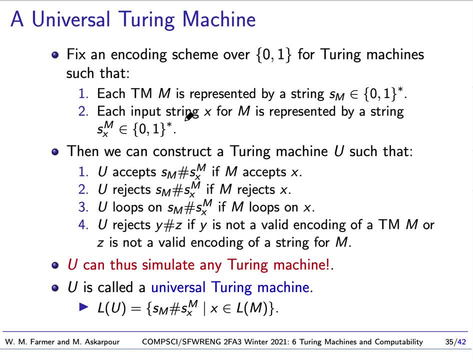 going to need a way of encoding Turing machines as strings over zeros and ones, And if we? if you go to Kozen's book, he describes how to do it, But there's a lot of ways this could be done. You could work out your own scheme. The scheme works. 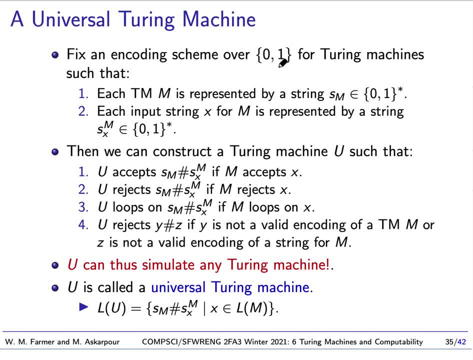 Because we only have a finite number of states, a finite input alphabet, a finite tape alphabet, a finite number of possible transitions and so forth. So we need a way of encoding up the whole description of a Turing machine as a string of zeros and ones. 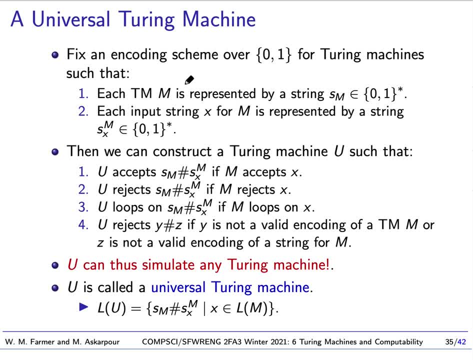 So we're going to assume we have a way of doing that. So let me ask this particular question. Sure, doing this, Like I said, there's many ways of doing it. So if we take a Turing machine, we will have a representation of it as a string. And not only that if we take an input string. 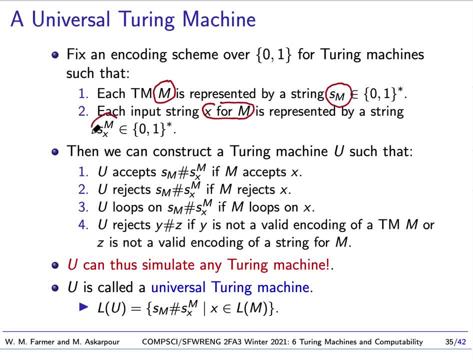 for my Turing machine. we will have a string that represents it, And now what we can do is construct a Turing machine. U and U takes strings of the form like this, And if the first part is a code for a Turing machine and the second part is a code for an input, 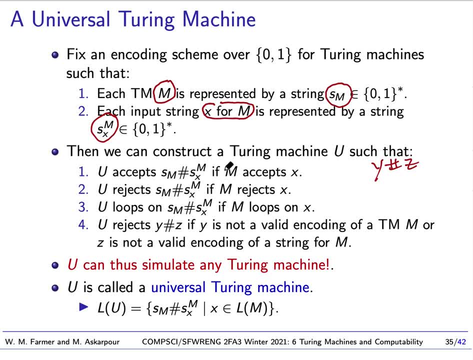 for it and U accepts that string, it will do it when M accepts X And it will reject that string when M rejects X And it will loop on that string when M loops on X. So U simulates exactly what M would do. So if U is running on this string, it will simulate. 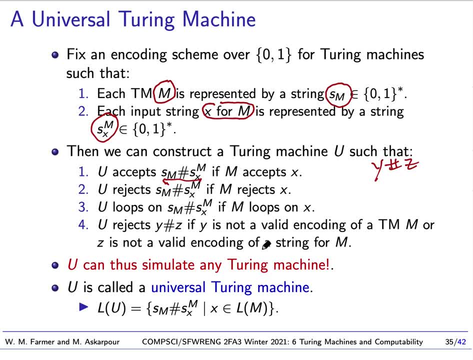 exactly what M will do on X. And if we give it a string YZ, where Z is the first string waiting megabyte And then Y is now the last string gem, You move around your line path right for X and then you type in 100,, 0,, YZ, YZ, where Z is not a valid encoding. 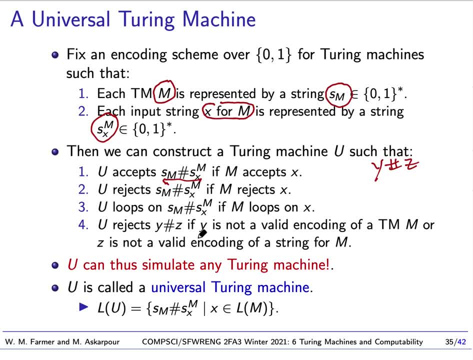 Then it will reject. So this is what U does, And we construct such a Turing machine U, And so this Turing machine can simulate any other Turing machine, So in a real sense simulate any Turing machine with it. So this is called a universal Turing machine, And 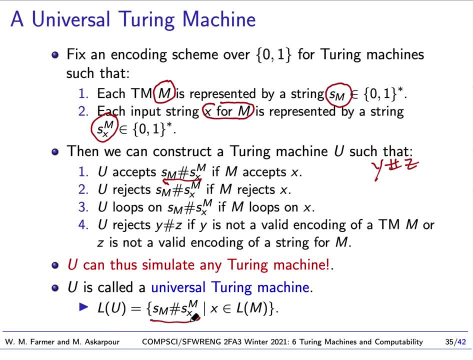 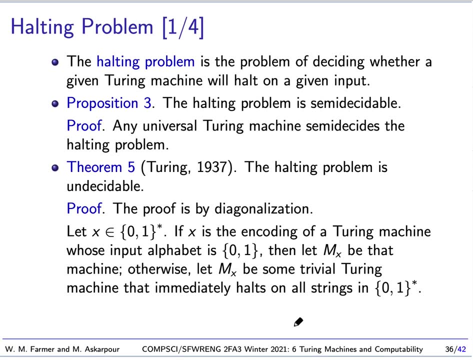 the language it accepts is going to be the language of strings of this form, such that x is a member of the language accepted by m. Okay, so now let's talk a bit about a very important problem: the halting problem. So this is a problem of deciding whether a given Turing machine, m, halts on a given input. 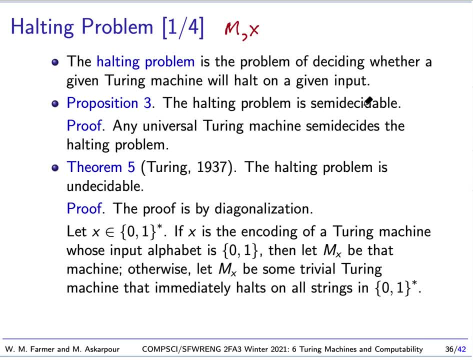 x. Now we know this problem is semi, we know it's semi-decidable. This is easy to show because if we take our universal Turing machine and we give it a code for m and we give it a code for an input for m and then we run that machine if the machine 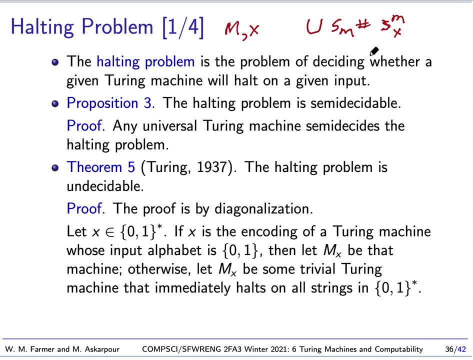 halts, then we know that m halts on x. Now the problem is: if the machine doesn't halt, we don't know if it halts. If it doesn't halt after a billion steps, it may halt after a trillion steps, but we don't know. 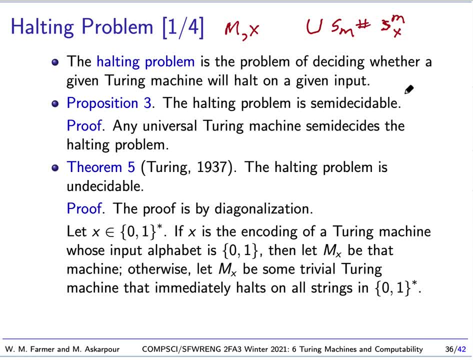 So that's why it's semi-decidable. It will answer the question, yes, if the machine, if m halts on x, but it won't necessarily answer the machine otherwise. So the halting problem, we can see, is semi-decidable. We know this by using a Turing machine. 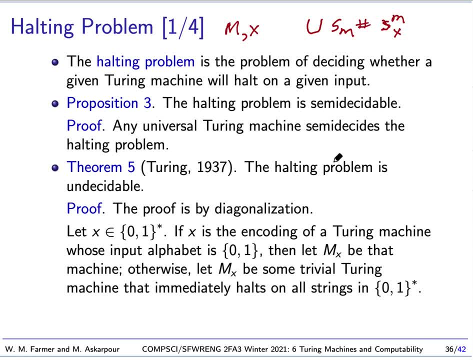 But it turns out not only is it semi-decidable, it is undecidable, And this is what Turing showed in 1937, and his proof is by diagonalization. So we're going to give the proof right now. Okay, so let's say we take any string of zeros and ones, Any finite string of zeros. 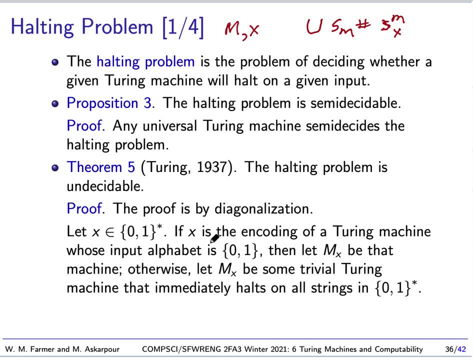 and ones. Now, remember, we have this scheme for encoding Turing machines. This string may be an encoding of a Turing machine. If it is, then we will say m is that Turing machine. So if x encodes a Turing machine, m says and so we'll accept that as well, And this will leave this thing. 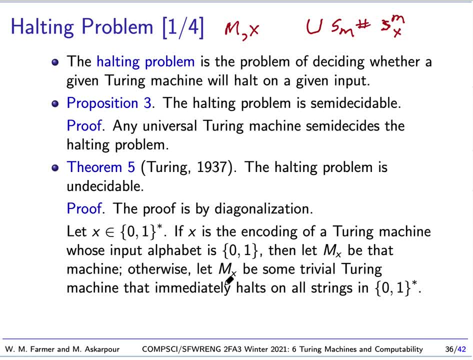 in this program. We can put this string in this했다 in any string of zeros and ones, In this case this string, because m is a Machine, Turing machine, m has to give 8歳 to the mx is that machine? If it's not an encoding for a Turing machine, then we'll say mx is. 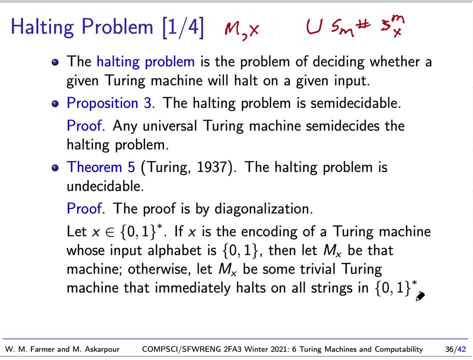 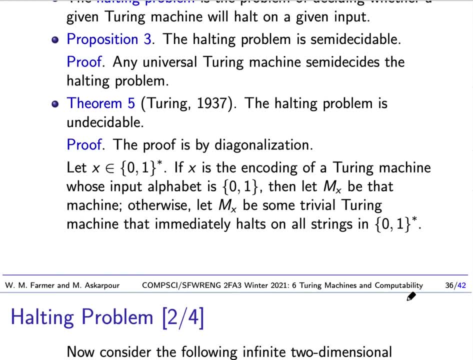 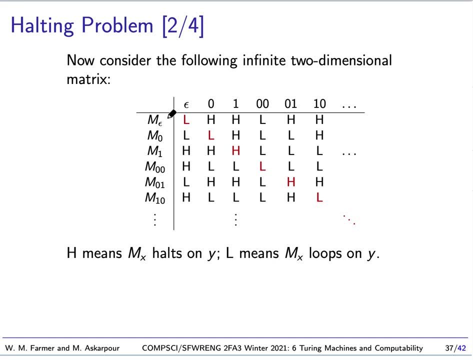 some trivial Turing machine that immediately halts in all strings. So you give it any string, it just halts immediately. Okay, so now let's consider the following infinite two-dimensional matrix. Over here we have all possible Turing machines and these Turing 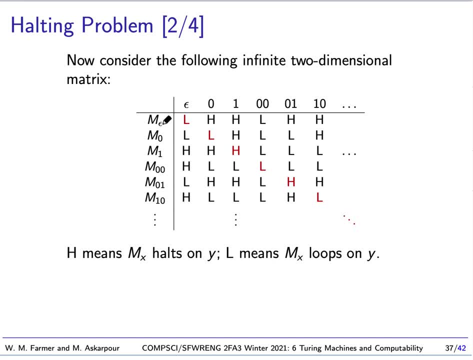 machines are given by are identified by strings of zeros and ones. Some of these are the trivial Turing machine that just immediately halts. Other ones are Turing machines that do something useful. And these are the possible inputs to the Turing machine. So these are remember. 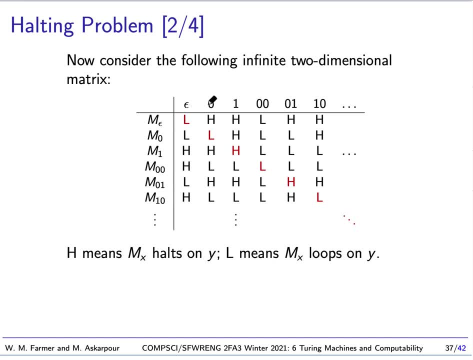 we're focusing on Turing machines that take inputs which are strings of zeros and ones, So these are the possible inputs. And then h here means it halts. So like if we look at this one and this one, this says: 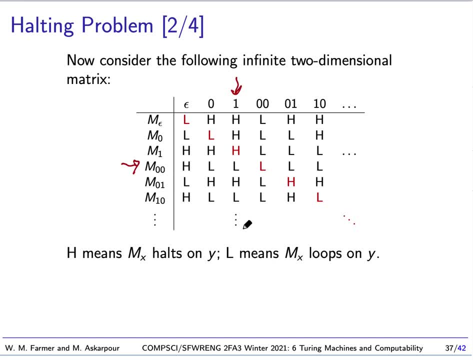 well, h means it halts, l means it loops. So this says that this machine, this Turing machine, given this input, loops. So we have this big, infinite dimensional matrix. We have all the possible inputs here, Okay, so what we want to do now is we want to assume that we have. 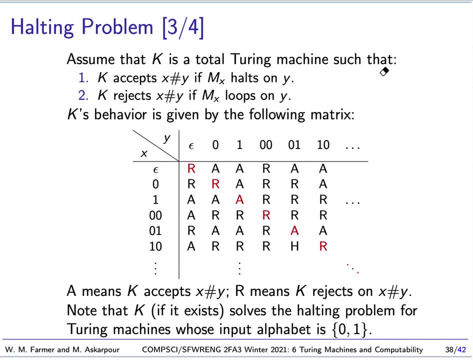 a machine, k. It's total And so it's a Turing machine. We're assuming that we have such a machine. It's total And k accepts x sharp y if the x Turing machine halts on y And it rejects x sharp y if the x machine loops on y. 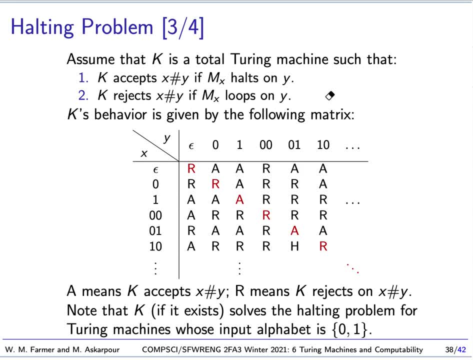 This is what it does. So remember halts. there's two possibilities: accepts and rejects. So this is we're assuming we have this machine And so we can describe the behavior using again this big thing. So for x we have possible strings. 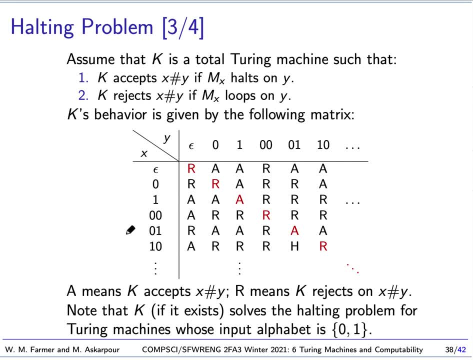 Y. we have possible strings If we look. if we have this as a string and this as a string, the A tells us k halts, And what that means is it means that M01 on 1, 0, I should say it means this accepts. 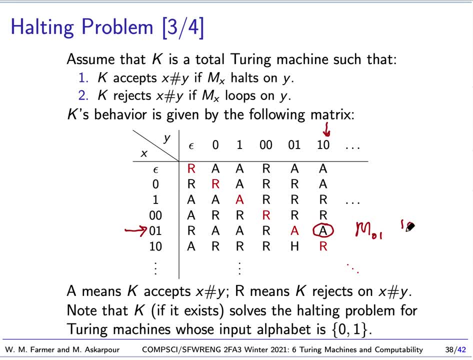 What that means is M01 on 1, 0 halts Okay, And for instance, down here we have a reject. That means that M10 on 1, 0 here loops. So this halts, this loops. 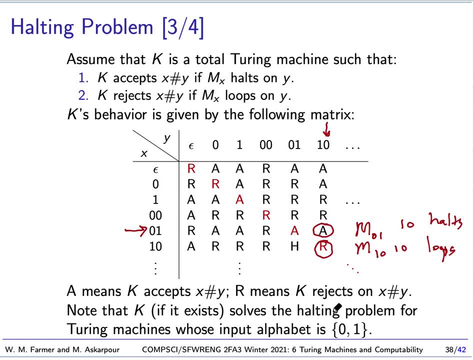 Okay, So that's what k does, And the important thing to note is that k solves the halting problems for Turing machines whose input alphabet is 01.. So it doesn't solve the halting machine for all, It just solves it for Turing machines with inputs alphabets consisting of 0 and 1.. 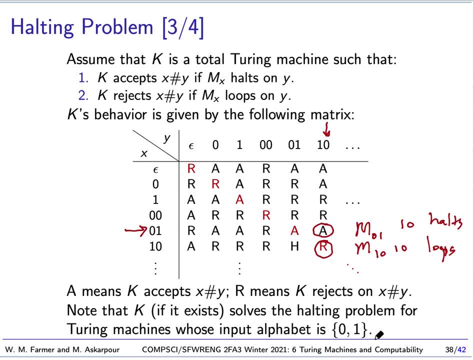 Okay. So what we want to show is that there can't be such a k. If we can show there can't be such a k, then we can't solve the halting problem. We can't even solve it for this restricted class of Turing machines. 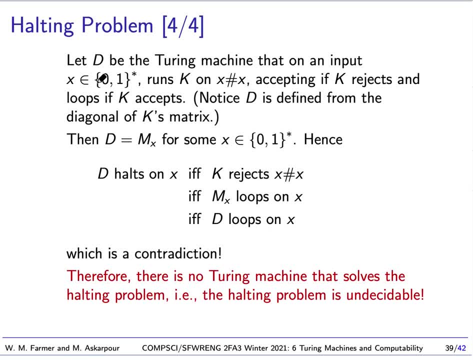 Okay. So what I'm going to do is: I'm going to create- I'm going to create- a Turing machine. d d for diagonalization. I'm going to use a diagonalization argument. I'm going to create a Turing machine. 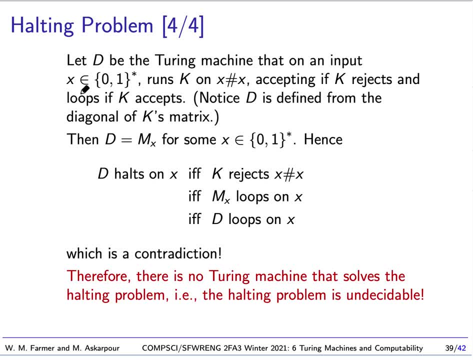 And this Turing machine takes an input, x, which is string of 0s and 1s, and it runs k. Remember, we have this thing I just described. We have this nice total Turing machine up here. We're going to run k on x, sharp x. 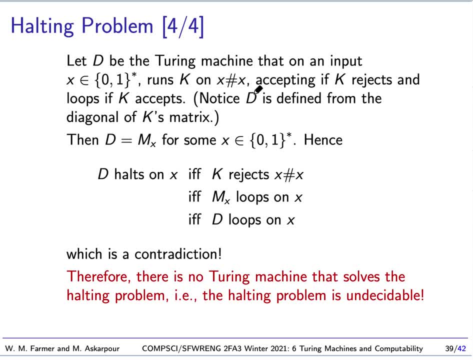 If you give it an x, we run k on x, sharp x. Now k will either accept or reject. Our machine will accept if k rejects and it will loop if k accepts. So this is pretty easy. If we have a Turing machine k, it's very easy to create this diagonalization machine. 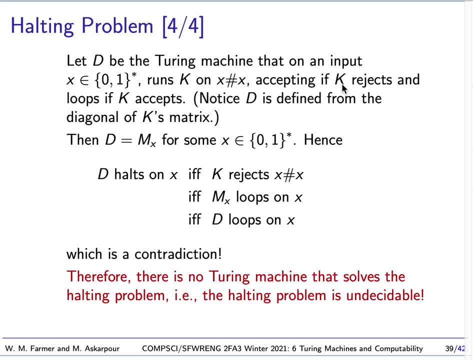 We basically can run k because we can simulate k Just the way we would with a universal Turing machine. So we can create this Turing machine And notice that the Turing machine is defined by the diagonal of k's matrix, Because what it does is if we were, when we're running k on this, this diagonal point xx. 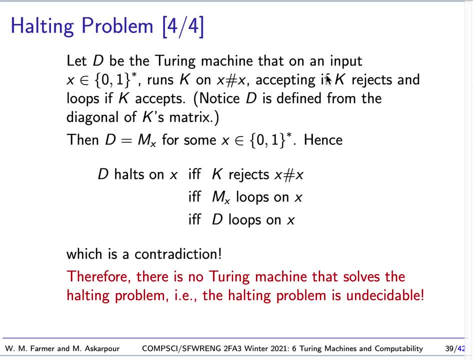 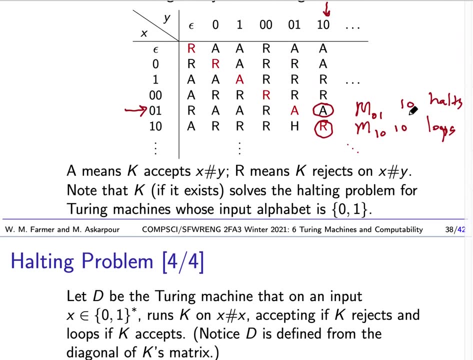 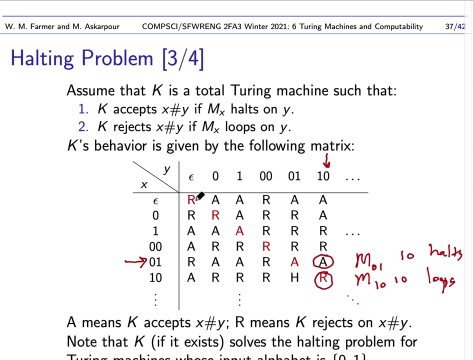 If k rejects, d accepts And if k loops. I should say if k accepts, d loops. So if we go up here and we look at the diagonal, If it rejects, we're going to loop. If it accepts, If it accepts. 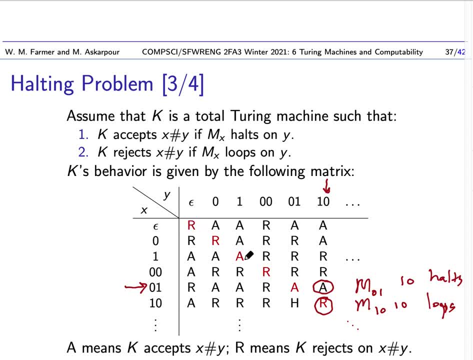 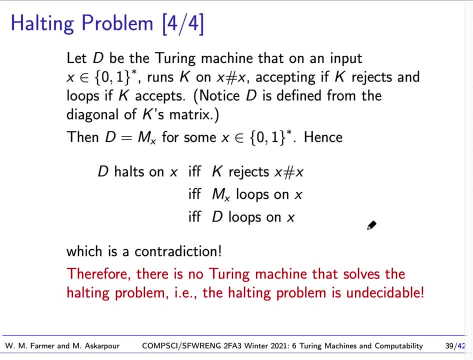 No, excuse me. If it rejects, We're going to accept, If it accepts, we're going to loop. So we change, We're going to basically change those. Okay, So we have this d Now. d is a Turing machine. 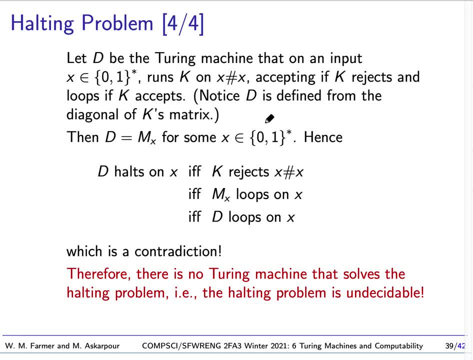 And we know from the Church-Turing thesis that it's like any other Turing machine. So it's going to have a code, And so d equals mx for some x. So there's going to be a code that goes with d. Okay. 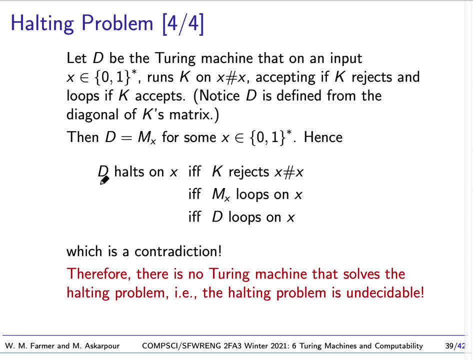 So now let's say we take d and we say that d halts on x. So this may be true or not, But if d halts on x, that's the same as saying that k rejects x, sharp x. That's the way d was defined. 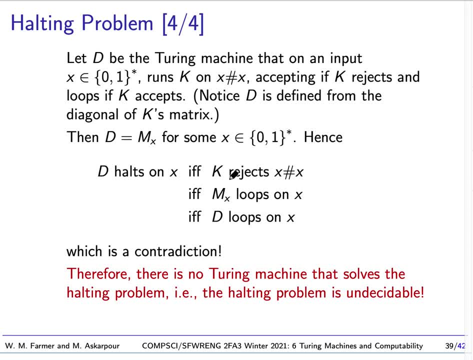 So d halts on x is the same as saying k rejects on x, sharp x. So k. what does k do? k rejects this precisely if the Turing machine for x loops on x. So this means mx loops on x. Now, mx is the same as d. 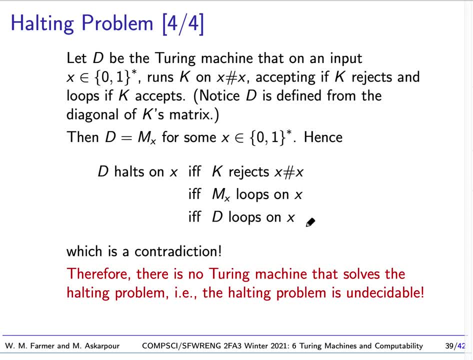 So this is the same as saying d loops on x. So what we see here is that d halts on x precisely if d loops on x. Well, this is a contradiction. There's no way a machine can both halt and loop at the same time. 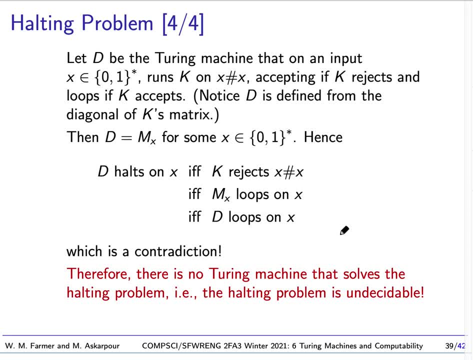 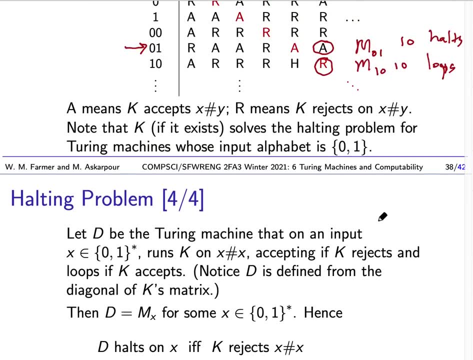 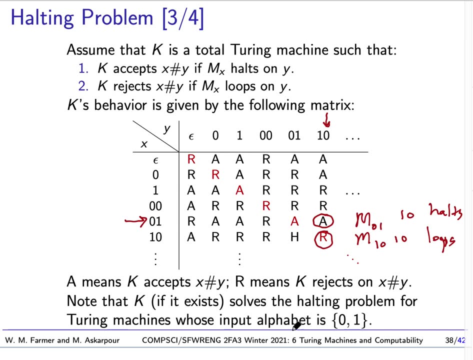 So this means there is no possible Turing machine k And as a result it is not possible to solve the. as I said here, it's not possible to solve the halting problem for Turing machines whose alphabet is 0,, 1,. 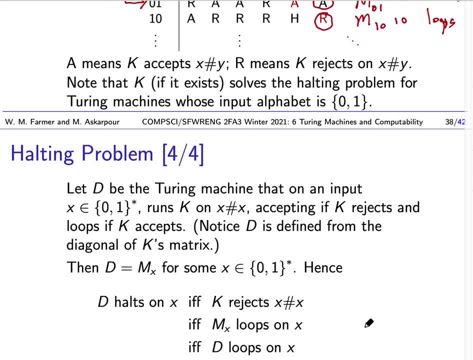 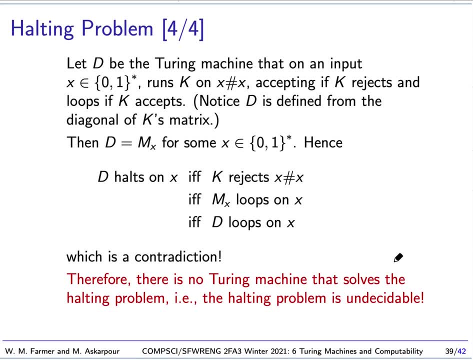 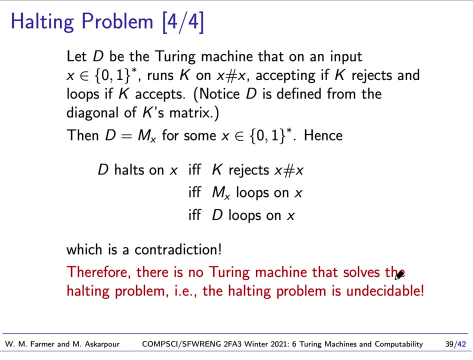 let alone solving the halting problem for all Turing machines. Okay, So this is one of the great theorems of theoretical computer science, one of the great theorems of computability theory, because it gives a precise example of a decision problem that is undecidable. 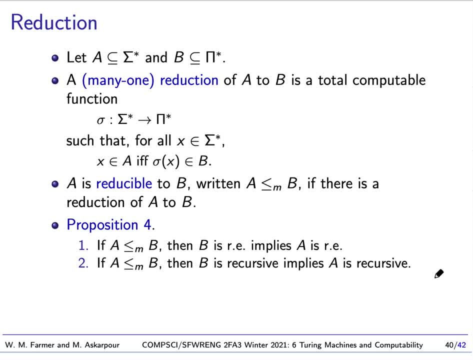 Okay, Now let's talk about something else. Let's say we had two alphabets, sigma and pi, And we have a set of strings of sigma and a set, I should say, a string a or set of strings a. 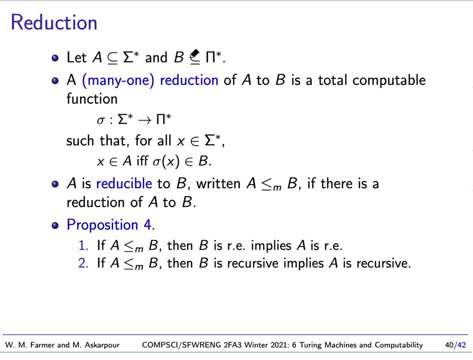 which are strings formed from the alphabet sigma, and similarly a set of strings b over the alphabet pi, And we can say that we have a reduction which is more precisely a many one reduction of a to b if there's a total computable function. 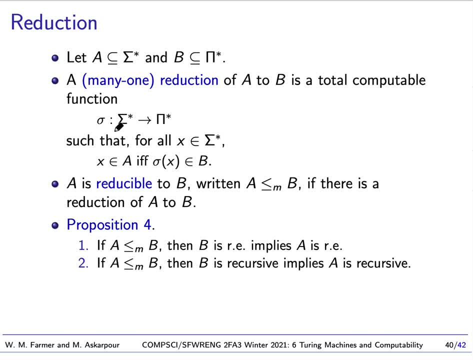 some total computable function that maps the strings of sigma to the strings of pi, such that whenever x is a member of a, that will be the case. that will be true if, and only if, the mapping of x, the mapping of x, is a member of b. 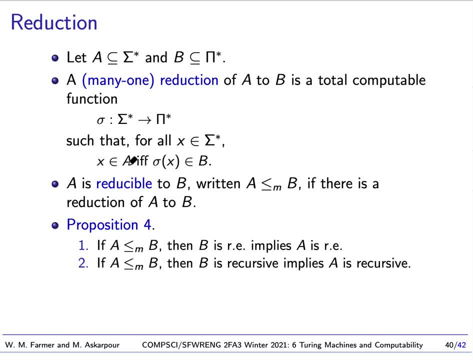 So another way of saying it, we can test whether x is a member of a by testing whether sigma x is a member of b, and vice versa. So this is so we say a is reducible, which we write like this: 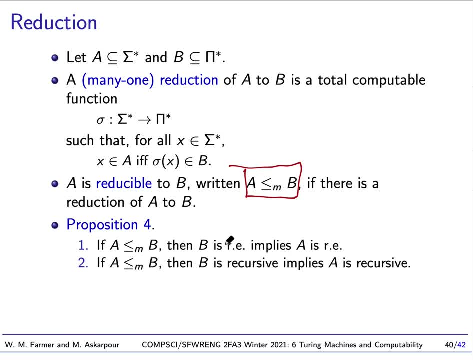 if there is a reduction of a to b, And what this gives. if you take a little time to think about it, it basically gives us the following theorem: If a reduces to b, then b is re. implies that a is re And similarly. 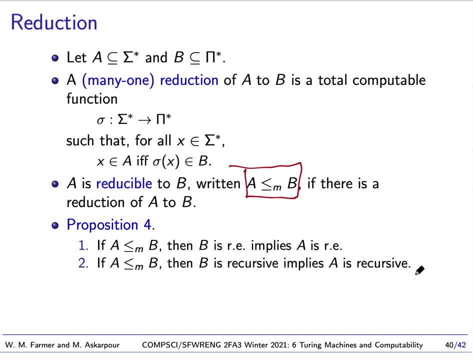 if b is recursive implies if a is recursive, Because basically the idea is, if we have this reduction and we know how to enumerate b, we can enumerate a by taking members of sigma star, mapping them to members of pi star and then seeing if they come up in the enumeration of b. 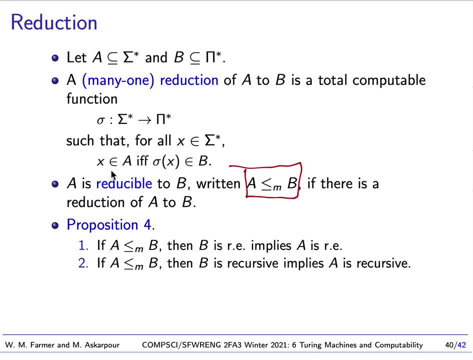 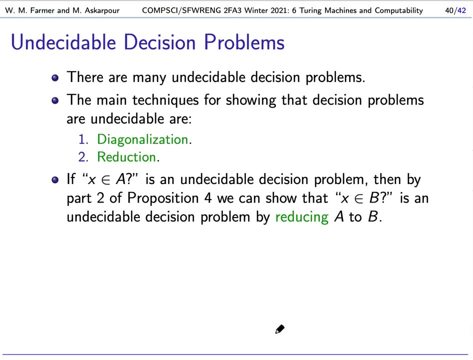 And they're going to come up in the enumeration of b only if they were members of a. Okay, so I won't go through the proof of the second one, but it's similar, So this is very useful because this means this gives us another way of showing. 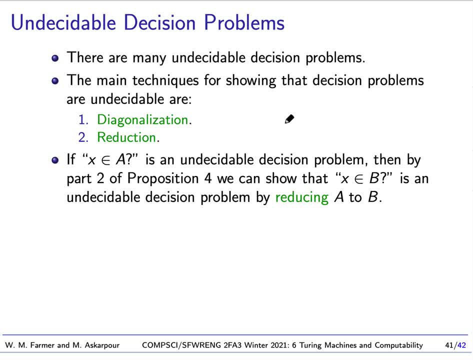 that there are undecidable decisions. So there's many, many undecidable decision problems And there's two basic techniques: Diagnostication, which we saw that we proved the halting problem is undecidable, and reduction, And the way reduction works. 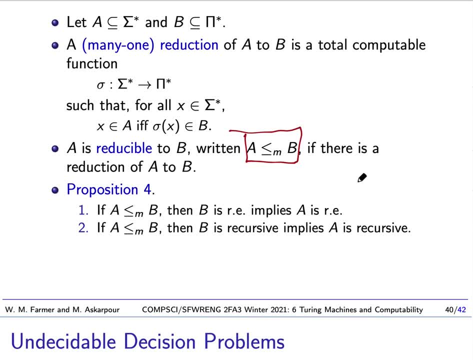 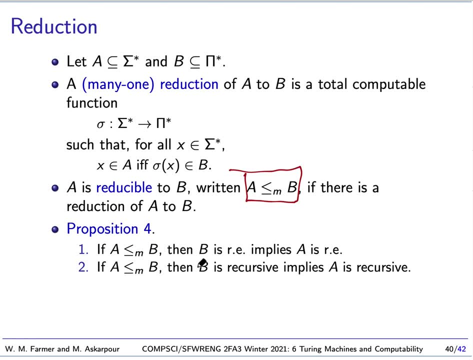 is, if you look at these theorems with reduction, we want to show that something's undecidable. What we want to do is take. let's say, in this case we want to take the contrapositive, which will be equivalent. 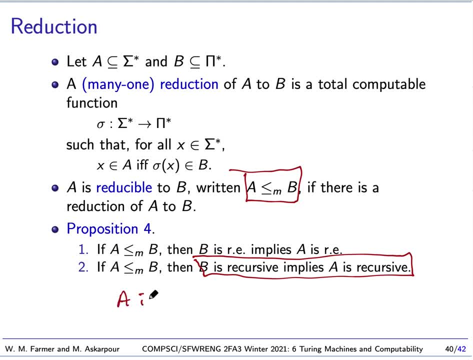 So we want to say: if a is not recursive, that implies b is not recursive. So let's say we were trying to show that b is not recursive. What do we do? We come up with a decision problem that is not recursive and we reduce it to b. 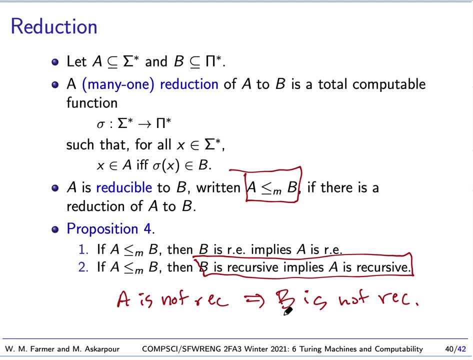 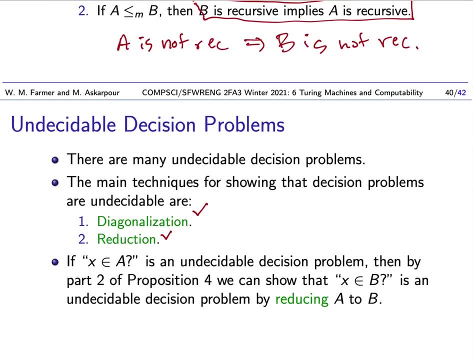 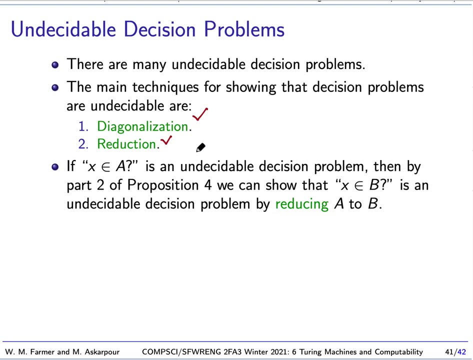 So this gives us another technique to show that decision problems are undecidable. So diagonalization gets us going, but reduction allows us to show that there are many, many undecidable decision problems by reducing undecidable decision problems to new problems. 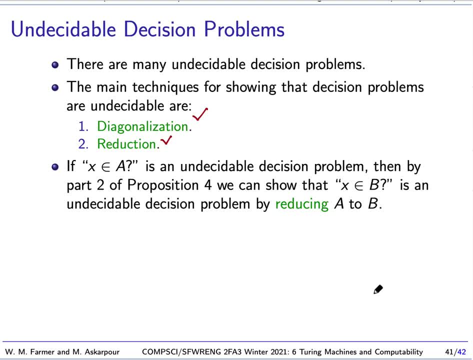 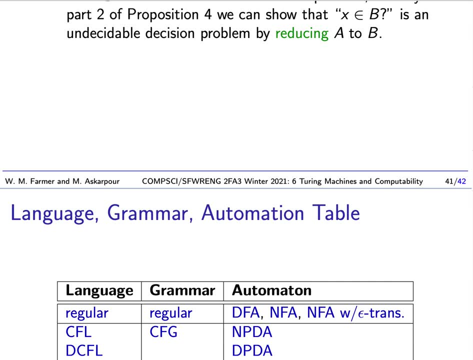 and thereby showing that those new problems are also undecidable. Okay, so we have one more thing which it looks like. I didn't have an end slide, so I can't quite show this, But the last slide which you'll see in the slides. 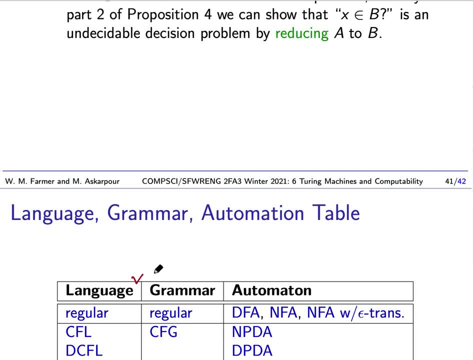 it shows a table that you've seen before of languages, grammars and automata And we have: we have regular, context-free, deterministic, context-free, linear, context-sensitive, re and recursive. So take a look at the slides. 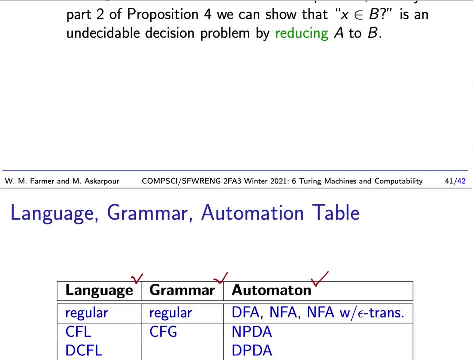 and you can see that. So this ends our lectures for this course. I hope you enjoyed them And that's all. Hopefully I will run into you later, Goodbye.